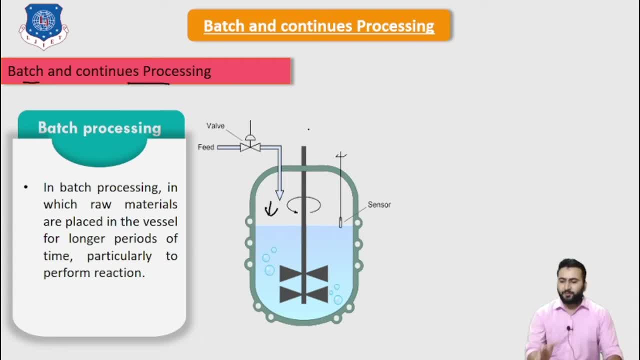 method. So in batch processing we are going to add raw material for the long period of time to perform reaction. To understand this, let's consider this reactor. Now let's suppose there is a two reactant, reactant A which has 80 kg and reactant B which is a 50 kg. So we are just 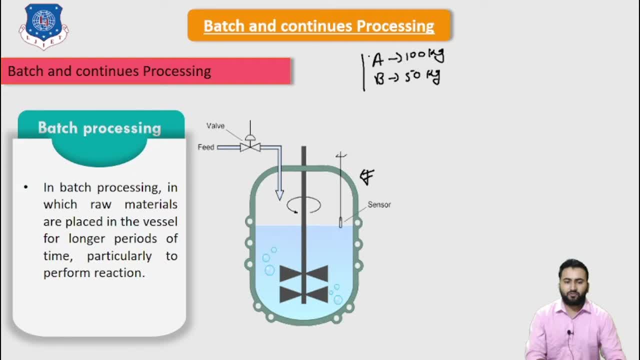 going to add this, both reactant, Directly into this reactor. Now we are going to allow this, both reactant to long period of time for the reaction and get produced the product. So this: both are allowed to settle down in this vessel and react with each other for long period of time and it 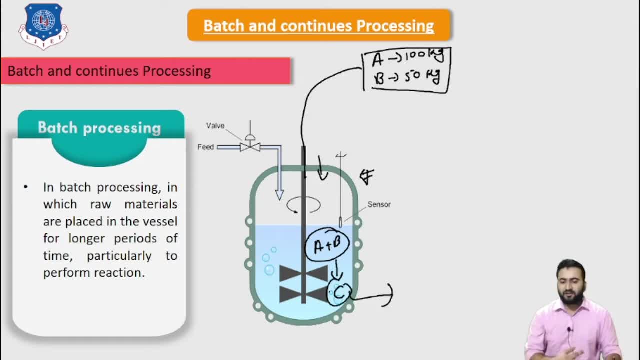 will be give product C After generation of product or after. let's suppose it will take two hours for the reaction. So we will take the product out from this reactor after the two hours, Right? So this is about the batch process. Batch process refer. 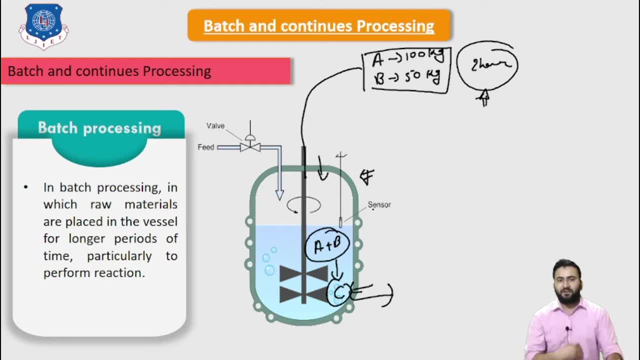 to a process that consists of sequence of one or more step that should be performed in definite order. The finite quantity of the product is produced at end of the sequence, Which is repeated in order to produce another product: batch: Generally, batch is a process. 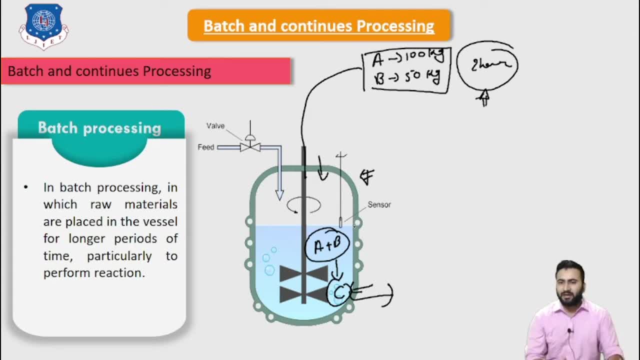 that result in production of limited quantity of material through a subjecting quantity of raw material to set of processing activity over significant period of time with use of one of more pieces of equipment. So the successive batches must be wait until the completion of current batches. Right, 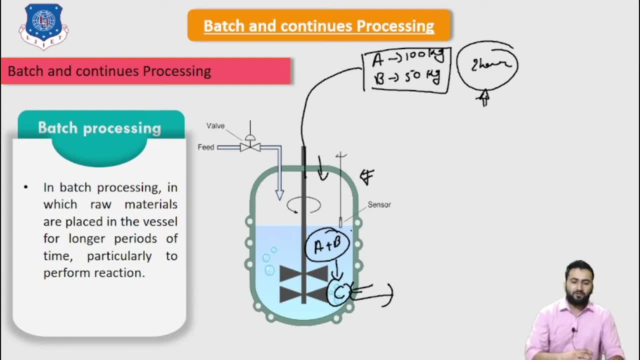 So if we are going to add some other chemicals or we want to produce other product, then we need to wait for certain time of period for the reaction. After that reaction and cleaning of this reactor, we can add another batch in this reactor. For that we are going to. 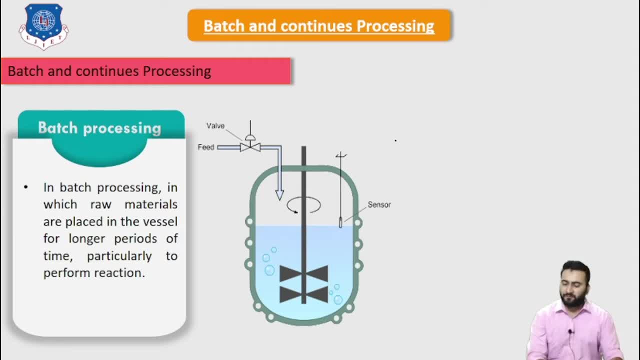 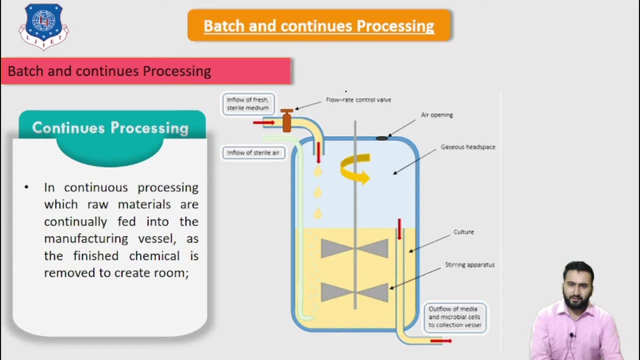 use bar chart for the scheduling this type of batches. Now let's discuss about the continuous processing. In continuous processing, which is raw material are continuously fed into the manufacturing vessel as the finished chemical is removed to create room for the reactantRightSo we are continuously removing product to create 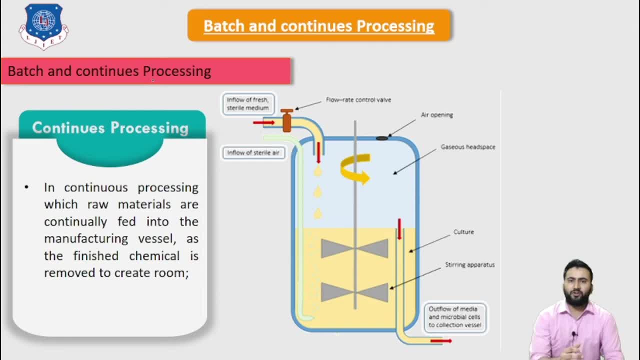 room for the reactant: A continuous process, So where a product that is made of raw material, which is continuously made of raw material, is removed to create room for the reactant. Right process, which refer to a processing that involving moving a simple work until at time between 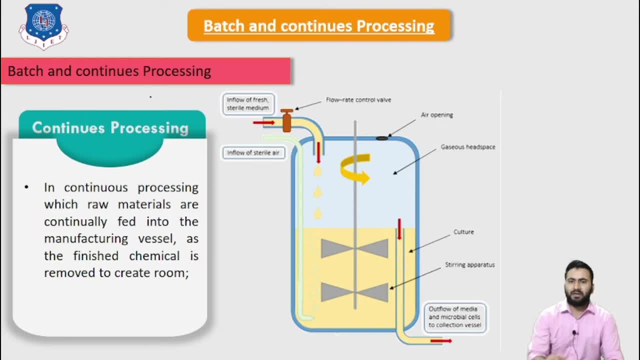 every step of process without break in time, substance sequence and extent. As the name suggest, continuous. so flow of product or material is a continuous. Every machine operate in steady state and perform certain process function. For majority of application, continuous flow save the cost or consider continuous process give better energy saving, time saving. 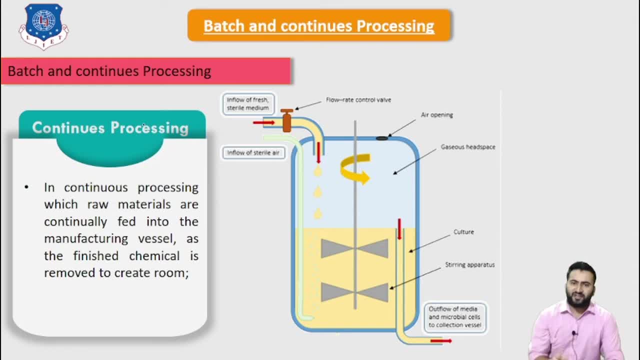 compared to the batch process. When this process is properly implement, it can reduce waste, improve quality by making it easier to identify and correct backfire the error, increase the productivity and adapt to a need of customer more efficiently compared to the batch processing. 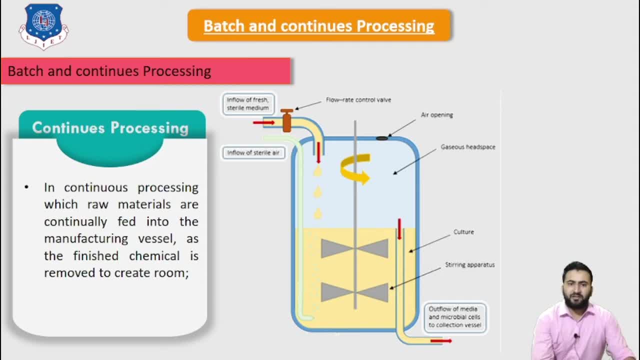 When comparing different process, the consideration always given to us advantages of continuous operation over the batch operation. In many case cost of continuous process is a reduced than the batch process or cost of continuous process is less than the batch process because in continuous process less. 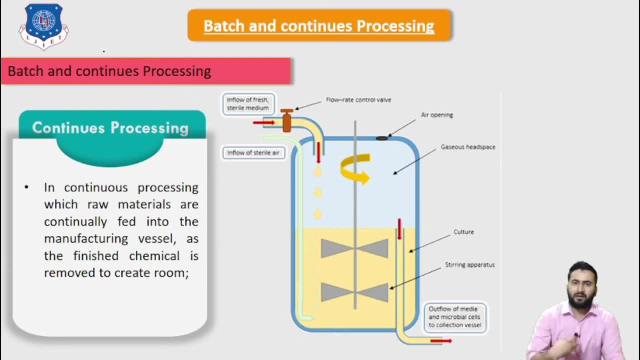 labor requirement and control of equipment and grade of final product is a simplified in continuous process. where in batch operation was common in earliest day of chemical industry, Most process have been switched completely or partially to the continuous operation right. So batch process is the 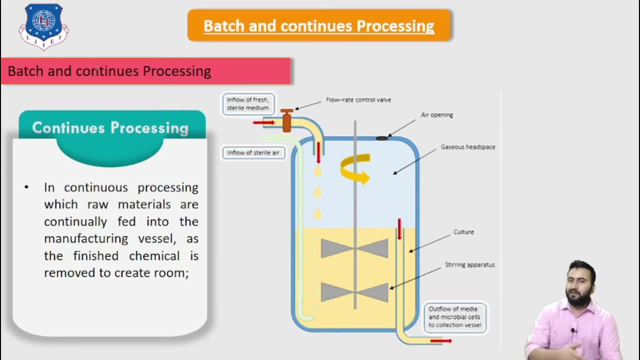 very old process and it's run in earliest days of 70s and 80s, which mostly converted into the continuous process or partially continuous process, which is a semi-batch process right. So evaluating advantage and disadvantage of every type of process is important to determine. 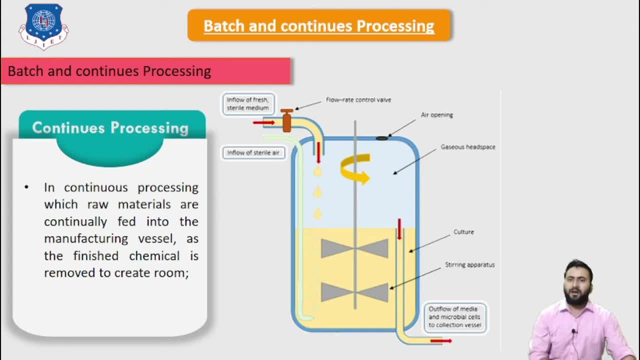 which one should be work based for the use. where it's come to the cost of equipment right, For example, the continuous process is most expensive than the batch process. However, when comparing the production rate with the batch process, continuous process is cheaper. one right: 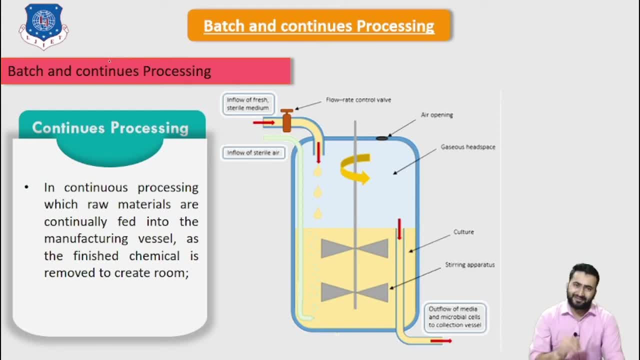 But absolute cost of continuous process is higher than the batch process. If you don't have enough manpower to perform the work, you can benefit more with the continuous process compared to the batch process. So if you don't have enough manpower to perform the work, you can benefit more with the continuous 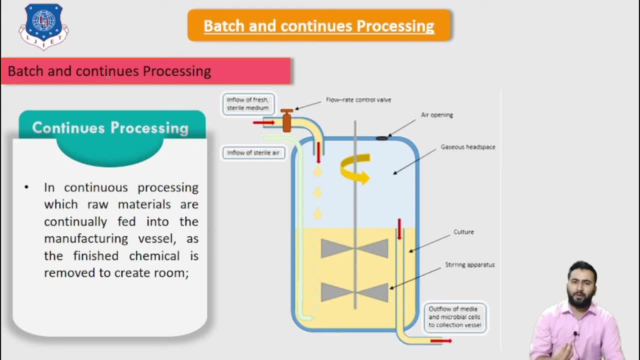 batch process because it requires fewer people than the batch process. In terms of ease of automation, batch process is relatively more difficult than the continuous process. Both continuous and batch process are vital in production of material or product. Having deeper understanding of each of them can help you make a inform about or taking. 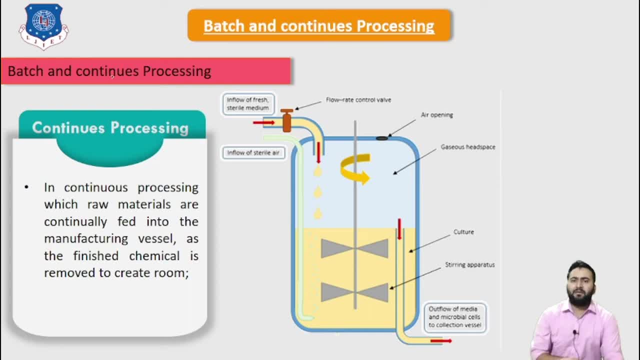 decision which one is the best. Plant having capacity greater than 5000 ton per year, then you should select the continuous process. But if plant capacity is the 500 per ton per year- sorry, 500 ton per year- then normally we are going for the batch process, right? 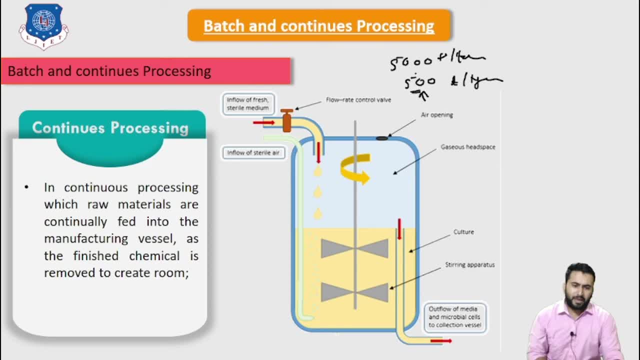 For less than 500, we are going for the batch For greater than 5000, we are going for the continuous process. To understand this, let's consider this figure. In this figure, we are going to continuously add reactant A plus B, right? 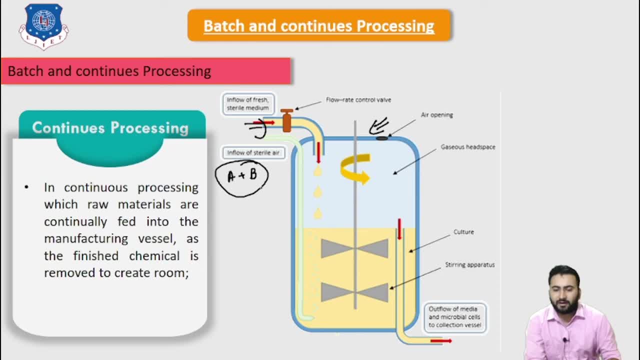 Let's take same example of batch process. We are here continuously going to add A plus B and reaction going to occurs and we are continuously removing the product. right, So we are going to continuously add reactant A plus B. So here we are continuously going to remove the product so we can continuously add the. 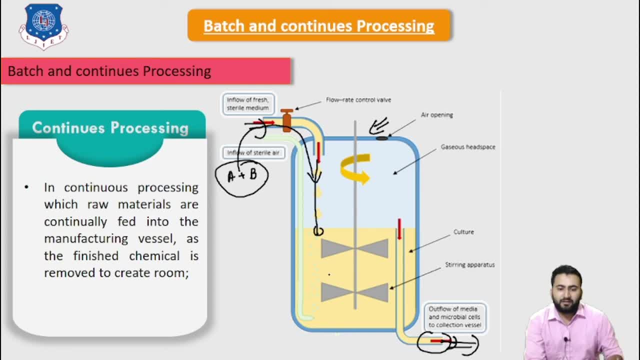 reactant, Because if we are going to react the, if we are going to remove the product from this side, it's create room for the this added reactant, right? So this type of process is known as a continuous process, right? 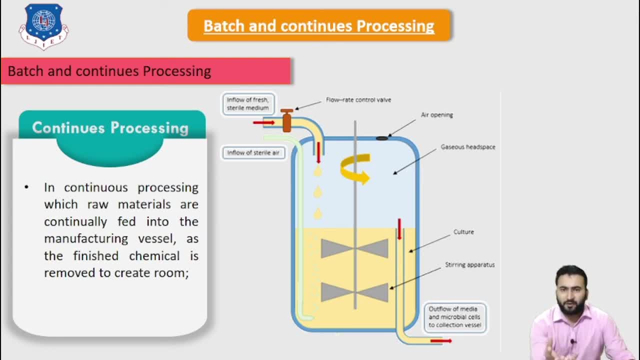 Now batch process are often preferred for the production process, So this type of process is known as a continuous process, right? So what we have seen from the product here, in product product we have very sort of a production process or building product odor production process. 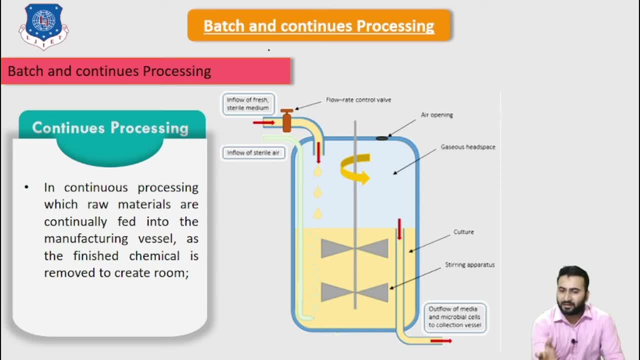 Now Batch process is available as a seasonal product. In General, Batch Plant are often preferred for the product which is as seasonal demand. So batch process has an advantage. When you you have a plant of seasonal product, then you can use batch process- chili Batch. plants are often preferred for the product with the seasonal demand. The greater ability of Batch Plant make them more sustainable for product with the short life time. Some reactions are so close that batch reactions are only sustainable without pages. Some reaction are so low that batch reactions are only sustainable. 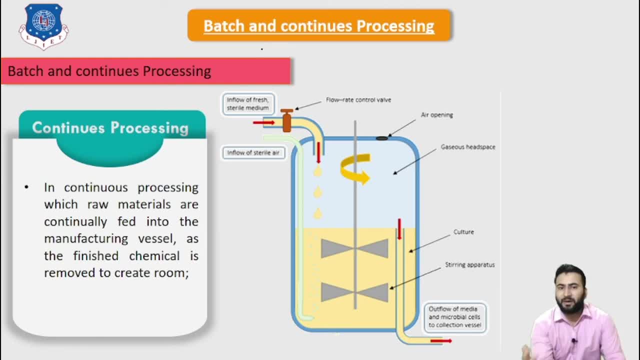 So plant 잘�era has算ok Left overmont Here. zero Zinc lifiton is a taueng étant present, The called vị �n activity. there is some salinity there, alternative compared to the continuous process, right. So if this reaction or if 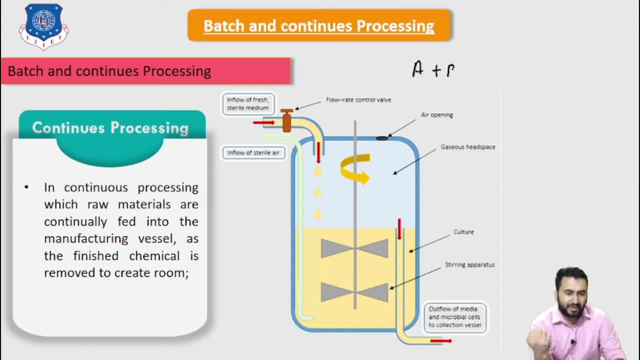 for this reaction. let's suppose this reactant A and B for this reaction and this reaction occurs very slow. if we are going to add this, both reactant and producing C, but this reaction takes too much time to produce C, then we cannot. 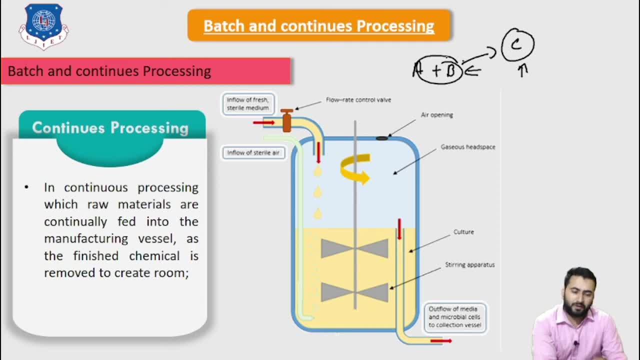 use the continuous process. We need to go for the batch process right. So it is very difficult to build continuous process when low capacity of slurry must be handled. So this is also disadvantage of the continuous process. if you need to handle a slurry which is in a low capacity, then we should go for the batch. 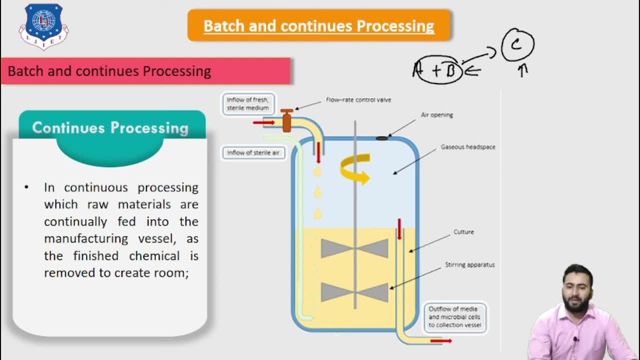 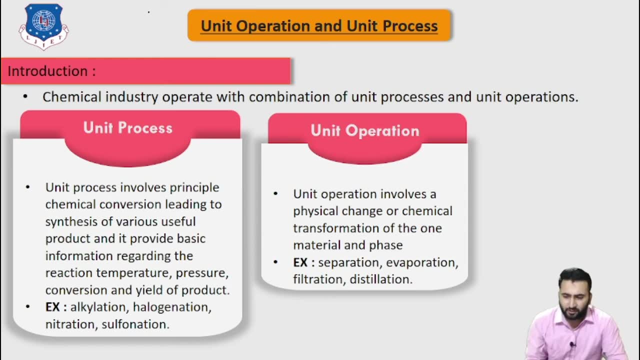 process right. So this is about the batch process and continuous. Now let's discuss about the unit process and unit operation. A unit process involves principal chemical conversion leading to synthesis of various useful products, and it provides basic information regarding the reaction, temperature, pressure, conversion and yield of product, For example, alkalination. 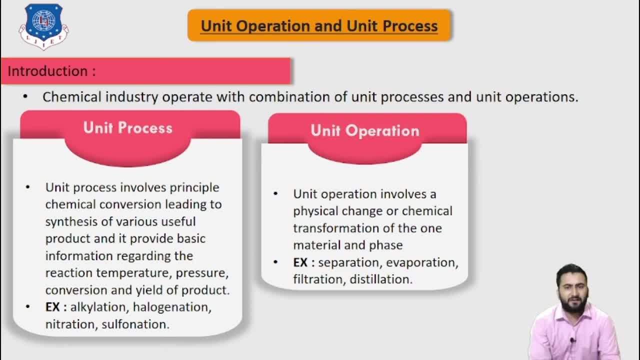 halogenation, nitration and sodium. Therefore, it is possible to use the group of two bioreactor in the unit process. Now let's discuss about the unit operation. Unit operation involves a physical change or chemical transformation of the one material and phase, For example separation, evaporation. 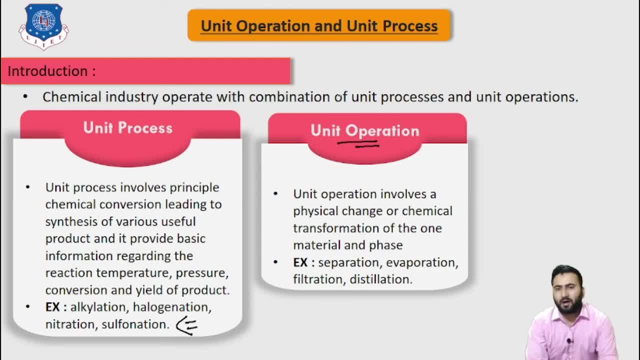 filtration, distillation. So this all are unit operation. Chemical industry operate with combination of two operations and the one process. right So when the chemical of unit process and unit operation. right. So in chemical industry any plant which 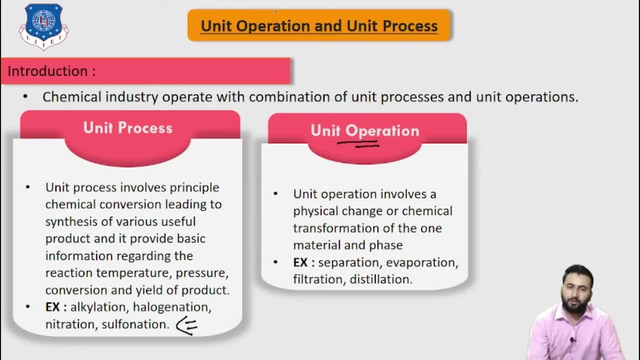 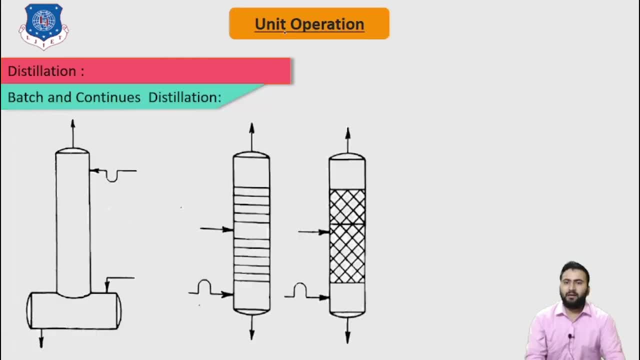 we are going to produce for any chemical it combination, it use combination of unit process and unit operation, right? So let's first discuss about this schematic, The. this schematic is used for the batch distillation. where this schematic are used for the continuous 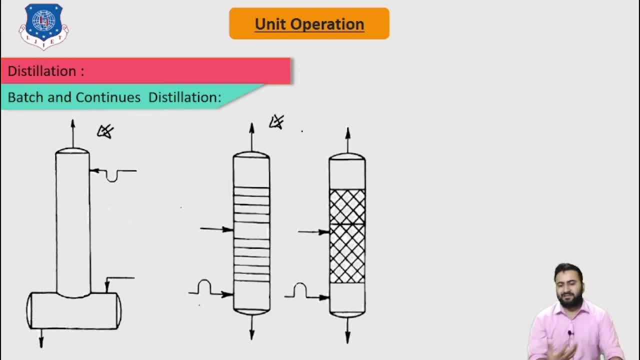 distillation process right. This schematic represents are important to draw the process flow diagram for the any chemical plant. Process flow diagram is the arrangement of all equipment for manufacturing of single product right. So to draw the process flow diagram we need: 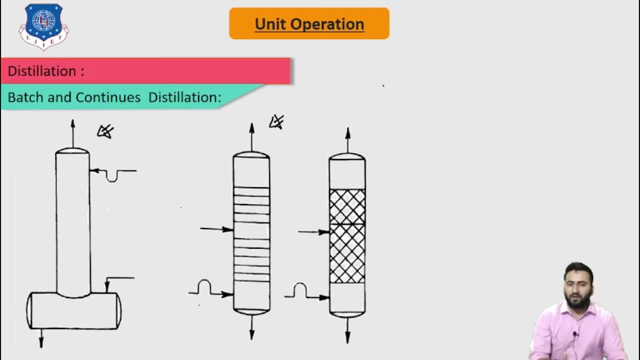 to understand certain symbol which are used for the particular equipment. So this is a symbol for the distillation, or can say that batch distillation, where this is a symbol for the continuous distillation. In continuous distillation. this is a tray tower where this